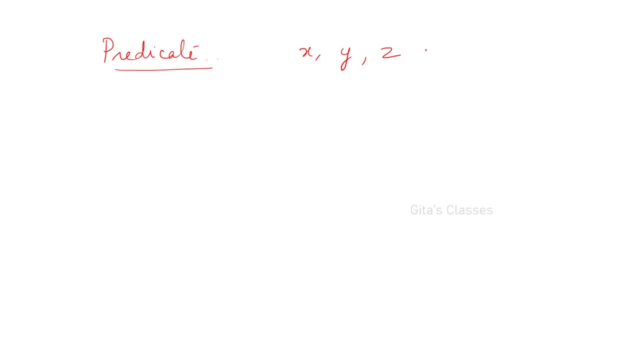 or statement. Suppose: if you have some xyz, some variables in the statements and if you assign some values to these variables, it will become a statement. Then it is called a predicate. These xyz are called variables. Then we can quantify these predicates, which is called quantifier. 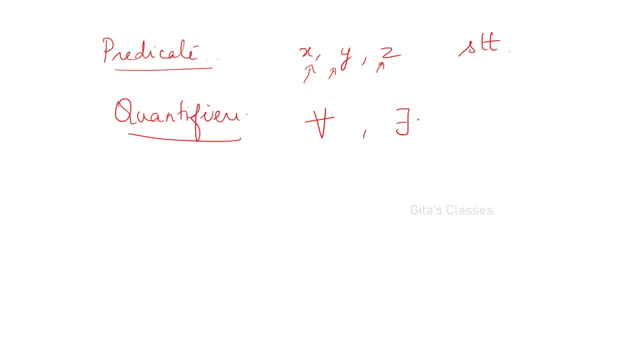 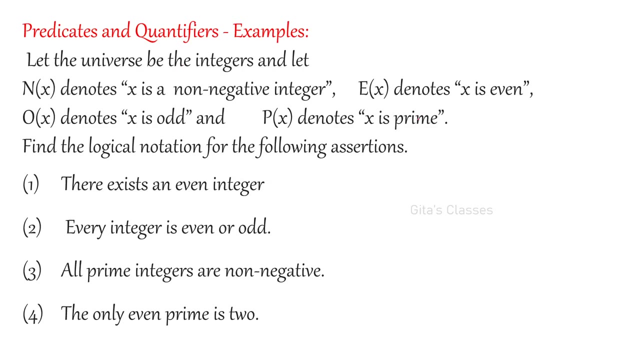 We have for all and there exist Two main quantifiers. we have seen for all and there exist. So if English statements are given, we can write in symbolic form, and if symbolic forms are given, we can write in English. Those kind of problems will be asked. So let the universe be the integers. 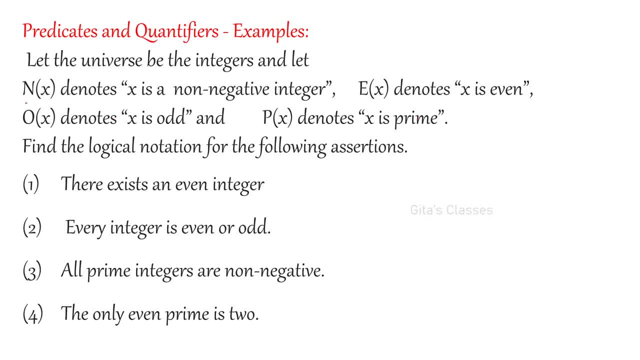 and let capital N of x denotes- This is the given question- N of x denotes x is a non-negative integer, E of x denotes x is even, and O of x denotes x is odd and P of x denotes x is prime. So we have to find the logical notation for the following assertions. First, 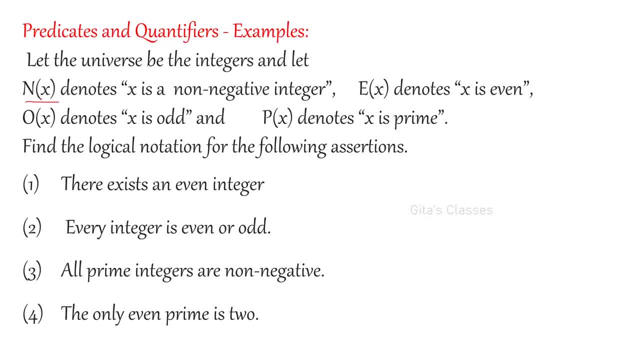 question. There exists an integer. Please remember N, capital, N is non-negative, E means even O is odd, integer. P is prime, So find the logical notations. So there exists an even integer. Even integer is what E of x? There exists an even integer. 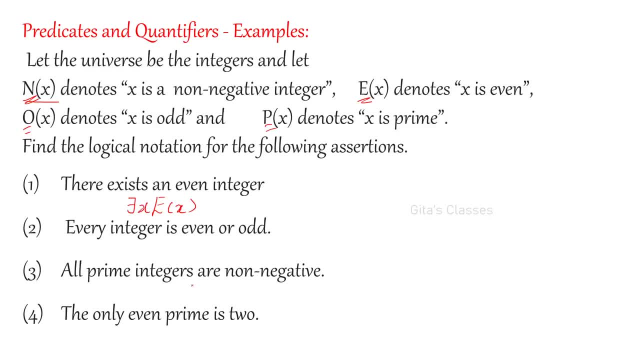 So there exists E of x, Very simple: Every integer is even or odd. So here, always remember, the universe is set of integers. For all these notations, universe x is taken from the integers, only Set of all integers. So universe of discourse is set of integers. So every integer. 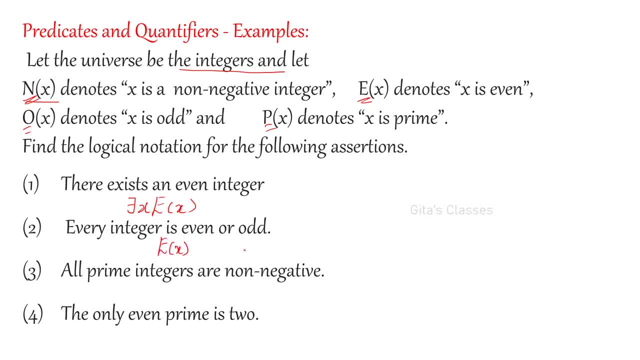 is even or odd. We know for even E of x or O of x, Either E of x or O of x. So we have E of x or O of x, Which one? All the integers are either E of x or odd of x. So E of x is. 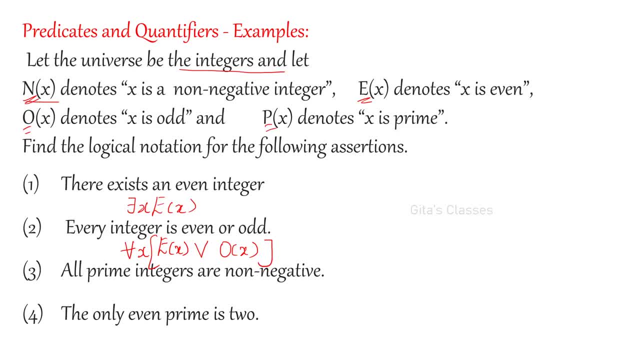 even O of x is odd and every integer is even, So this is for all x. This indicates that every integer, So for all x. either it has to be even or it has to be odd. Now, all prime integers are non-negative. All prime integers are non-negative. All prime integers are non-negative. 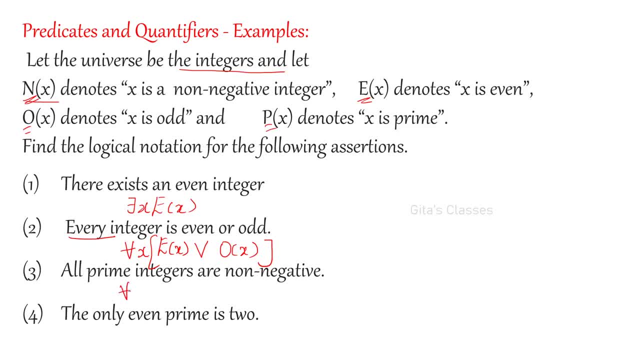 So here also for all x. Here we have to write all prime integers. Prime integers means P of x, and non-negative means N of x. Can you write here R or AND? We can't, because here if you take any integer it is given even or odd. Here all prime integers are non-negative. 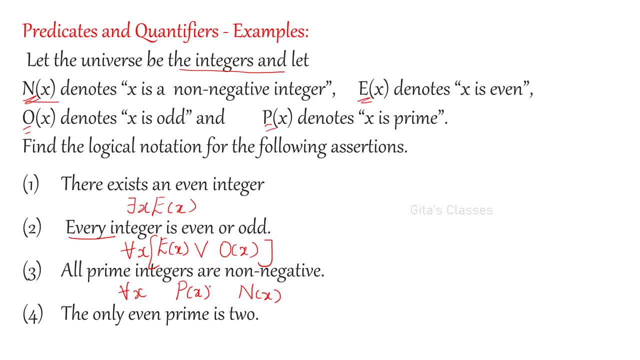 So if you choose one prime integer, it has to be non-negative. If you select prime integer, it is non-negative. That means if P of x, then non-negative. So this is a conditional statement For all x, For every x in the set of integers. if it is a prime, then it has to. 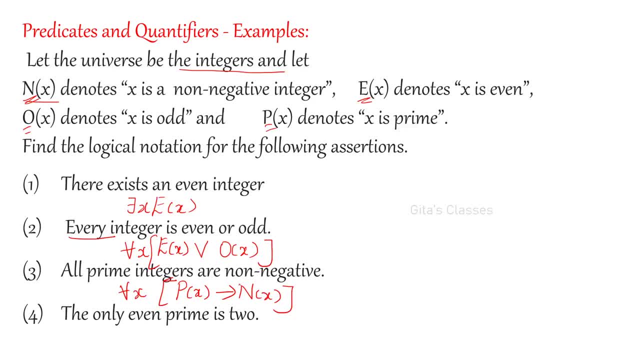 be non-negative. This is the given statement. And next is there is only one: only even prime is 2.. Only even prime is 2.. So if you take E of x, the only even prime is even number is x and P of x. So what is the condition? 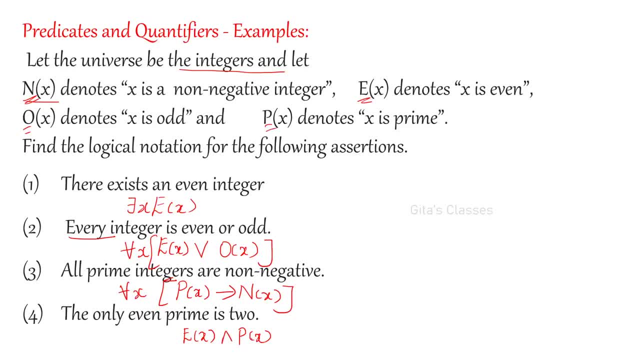 It has to be even and it has to be prime. Then if this is taken, So if you choose one integer which is prime and even number, it has to be 2.. So x is equal to 2. It has to be 2. Only possibility is 2 here. So every integer from the set of integers, 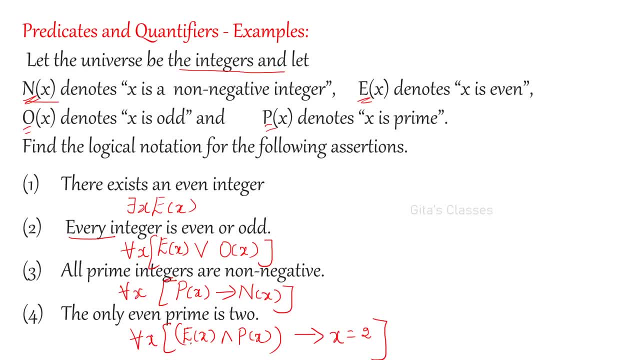 if you take for all x. If you choose one x which satisfies these two conditions, If it is even and prime, then it has to be 2.. So if you choose one x which satisfies these two conditions, then it has to be 2.. Only possibility is 2.. Therefore, E of x and P of x, then x is equal. 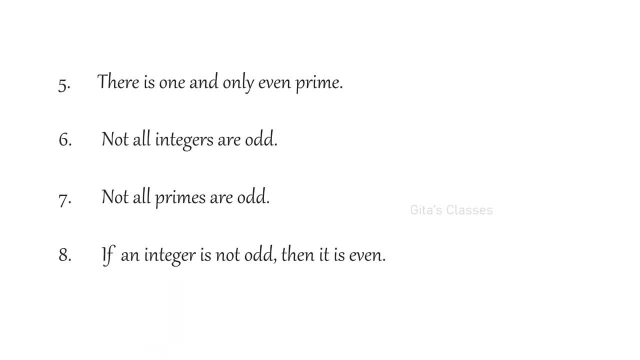 to 2.. Very easy. Only thing is we have to think and write, That's all. Now, there is one and only even prime. There is one and only even prime. So, apart from for all- and there exists- we have studied one more quantifier that is unique quantifier. So there exists. 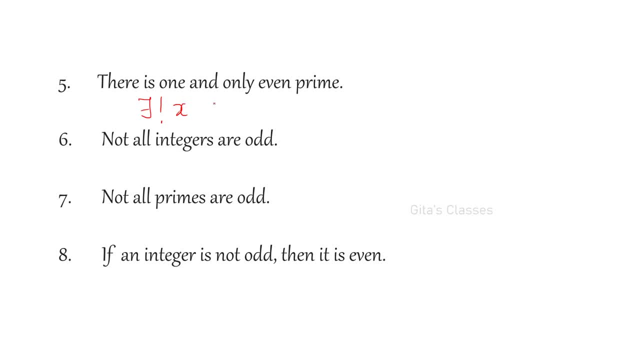 a unique value, x, such that it is even and prime. Now we are using that unique quantifier. Next is: not all integers are odd. Not all integers are odd. Not you keep it aside. All integers are odd. How will you write odd? Odd means O of x. All integers are odd means. 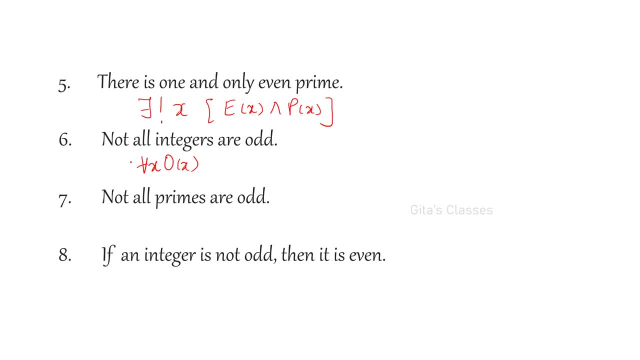 for all: x, o of x, Very simple. Take negation: Not all integers are odd, Simple. Or if you take this negation inside, what will happen? For all will become: there exists right, There exists x, not of o of x. This also can be done. Either you can write like this or write: 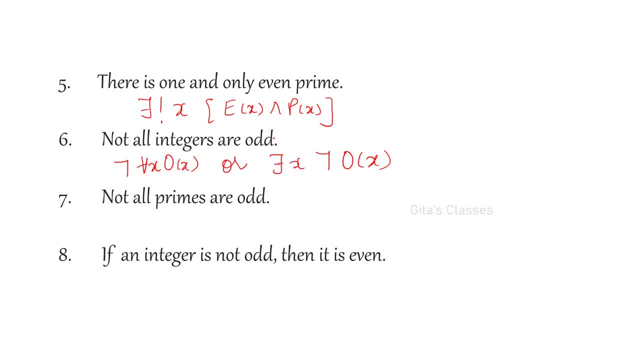 like this: There exists, not all integers are odd. There exists at least one integer which is not odd. That is also another meaning. Now, not all primes are odd, Not all primes are odd. So first you consider: if there is a prime number, it has to be odd number. 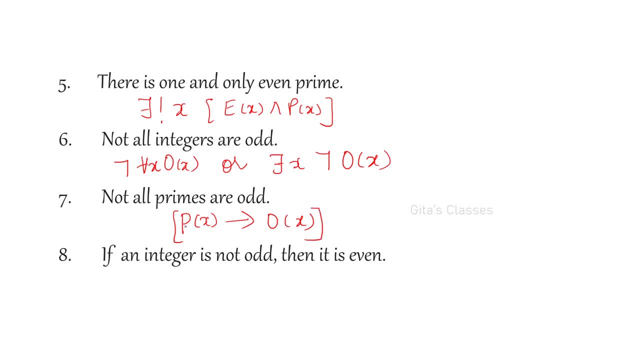 This is for all x, For all x. if there is a prime number, it has to be odd number. If there is a prime number, then it is odd number. right. But it is not true. There is at least. not all primes are odd. There are even primes also. We know that there is at. 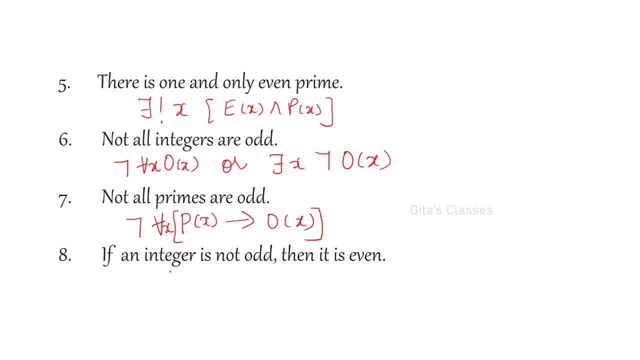 least one, even prime. Similarly, if an integer is not odd, then it is even Integer is not odd. Odd means o of x, not odd of x. So if this is true, then it has to be even number, And this is true for all x. okay, If it is not odd number, then it has to be even number. 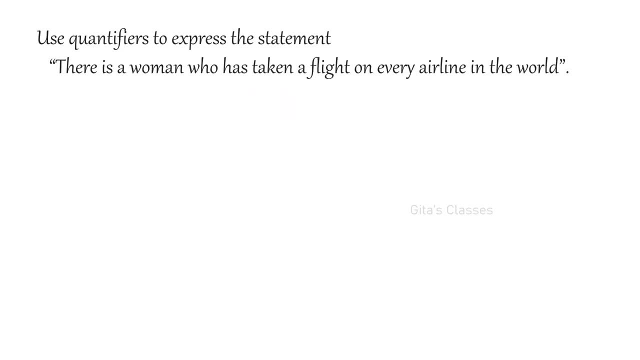 right. Next, use quantifiers to express the statement. There is a woman who has taken a flight on every airline in the world. So how can we write? There are two ways, and this is not unique way to write. There are two ways to write. There are two ways to write. 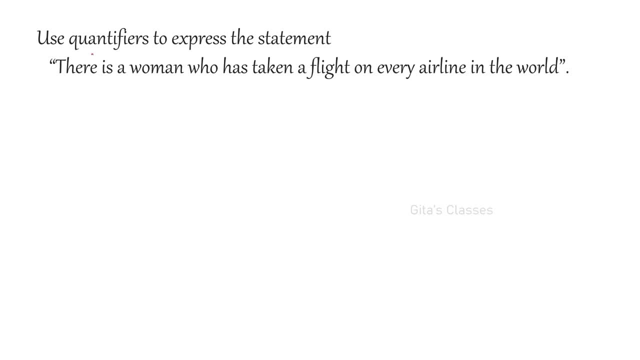 You can write your own statement also, So this is two ways I will tell you P of. we are having a woman, a flight and every airline, So let us take W, F and A. okay, So P of. 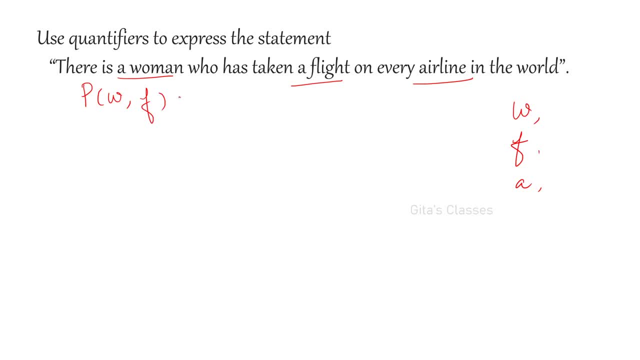 W F. A is the statement W has taken F, that is, woman has taken a flight. This is the statement P of W F, with two variables: okay, And Q of F. A is F is a flight, F is a flight on the airline A, So F denotes 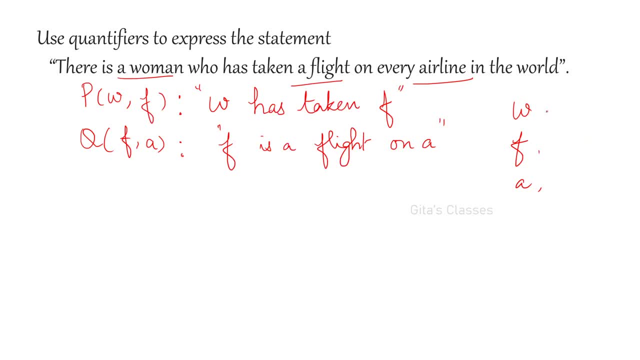 F denotes consists of all the women. okay, F denotes women, All the women, set of all women. and here F is set of all airplane flights, set of all flights, and A is all airlines. okay, These are the variables defined. These are the domain. 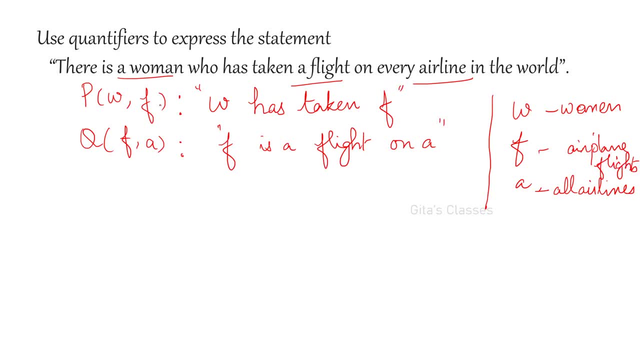 actually okay. So from now, these are the statements defined: W has taken, woman has taken a flight and F is set of all okay, So from now, these are the statements defined: is from this airline A right. But now, what do you want? There is a woman who has taken. 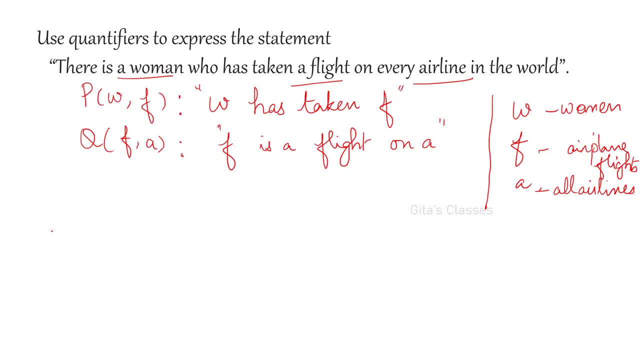 a flight on every airline in the world, right. So there exists a woman. there exists a woman, W, who has taken from all the airlines airplanes, okay, From all the airlines, from every airline, so for all A, from all airlines, she has taken at least a flight. So there exists F? P of. 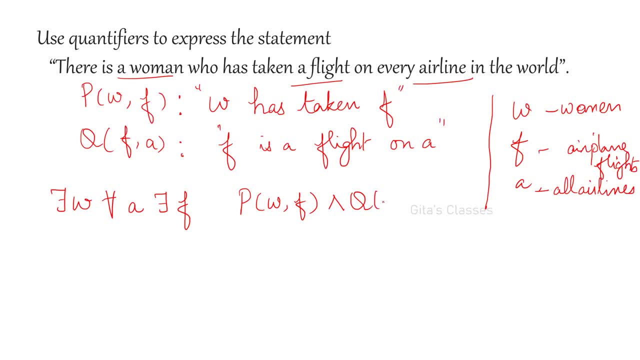 both has to be true: W, F and Q of F, A. This is one way of writing the statement right. Or you can even make it simpler, Or you can write- you can define all the three in a same quantifier, same predicate: the R of W, F, A. So W has taken F on A. You can directly: 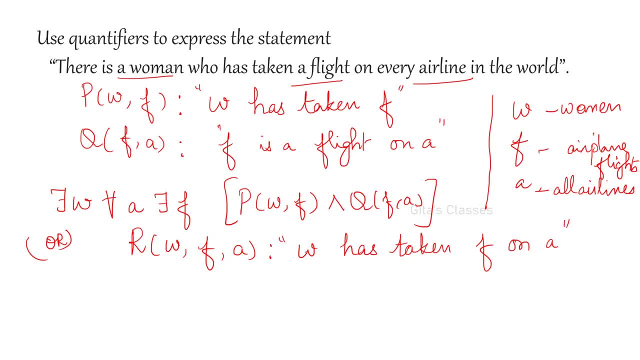 write this is actually simpler. okay, If you find this difficult, then you can go for 2, or you can simply write this one. Three variables also will be easier. Then how will you write here: There exists a woman, there exists W, the same for all: A. 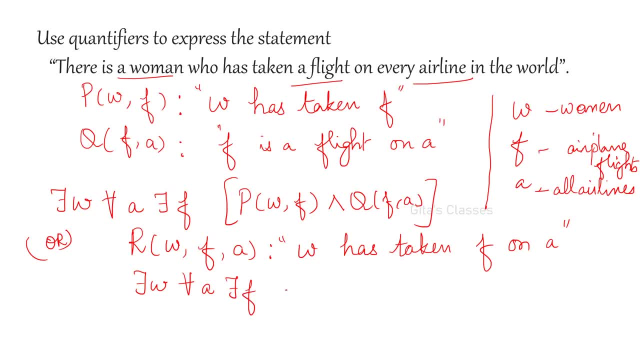 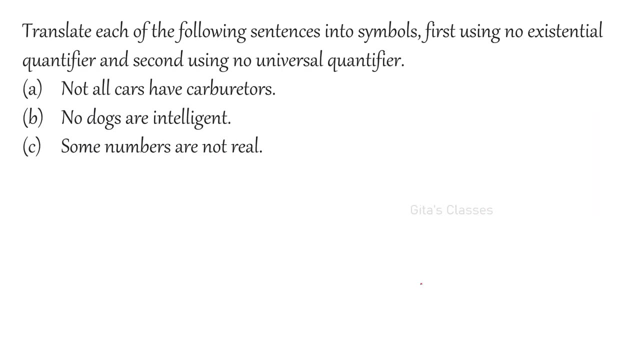 From all the airlines. at least she has taken a flight from every airlines. So R of W, F, A, Okay, any one. you can do Next is translate each of the following statement sentences into symbols: First, using no existential quantifier and. second, using no universal quantifier. 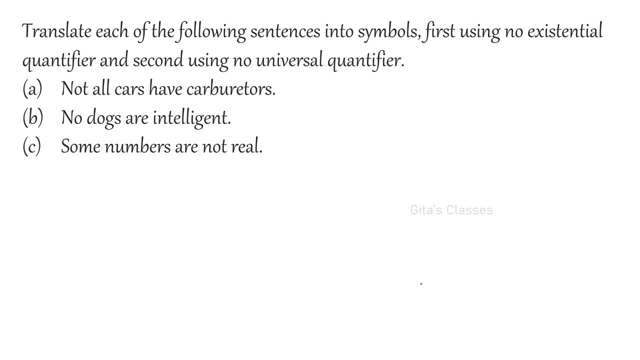 Okay, So you have to write. you have to write in two forms: One should not contain there exists, one should not contain for all. Okay, So universal quantifier, existential quantifier, is what There exists, right, There exists. X should not be there. And universal quantifier is for all, X, right. So in one statement: 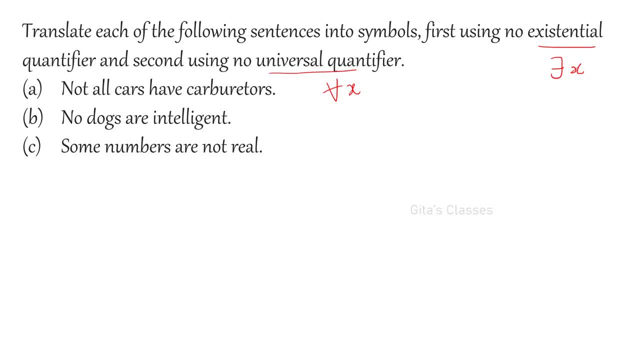 you have to write all these statements in two different forms. In one form: you should not contain, it should not contain there exists. In another form, it should not contain: for all X right. So that is what You read again. 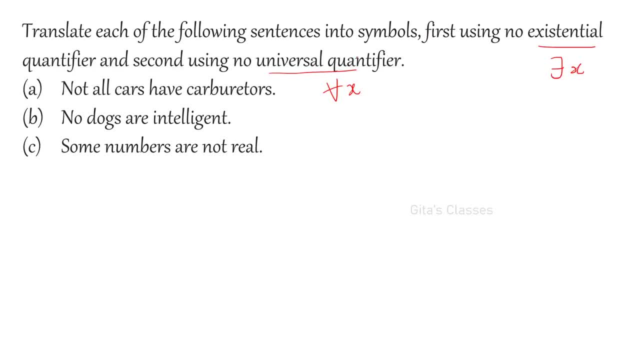 Translate each of the following sentences into symbols or symbolic form: First, using no existential quantifier and. second, using no universal quantifier. So first is not all cars have carburetors, right. So first one, let us define car of X, as X is a car And carburetor. 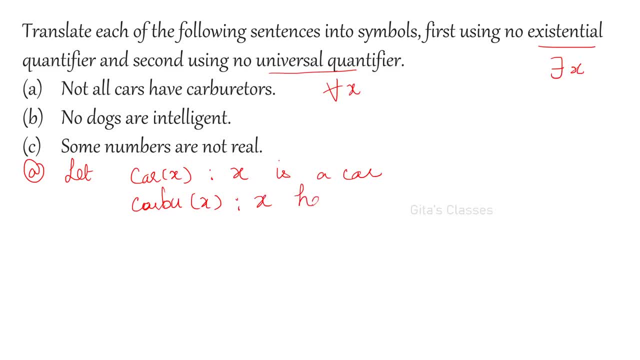 carbo of X is X. There is a carburetor, okay. So what is the statement? not all cars have carburetors, Not all cars have carburetors, So cars have carburetor. If it is a car, it will have a carburetor. 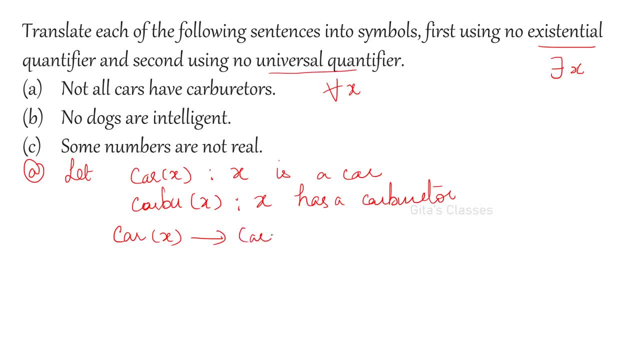 So if there is a car, then it will have a carburetor. That is the statement given right. Car of X, conditional carburetor of X. that is not All cars, not you, leave it aside. All cars have carburetors means for all x. 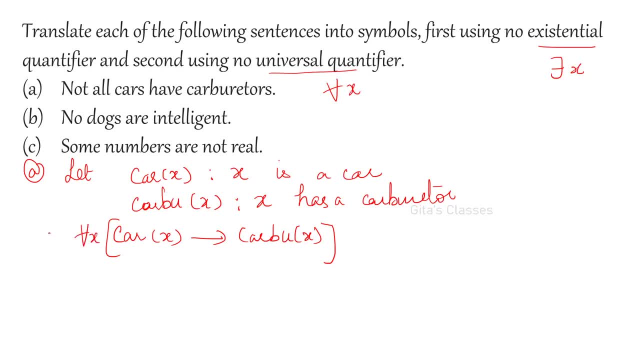 If it is a car, it will have a carburetor right Now, not you include that, not. So in one form we have written: that is here using for all x and there is no. there exists right. This is one form right. 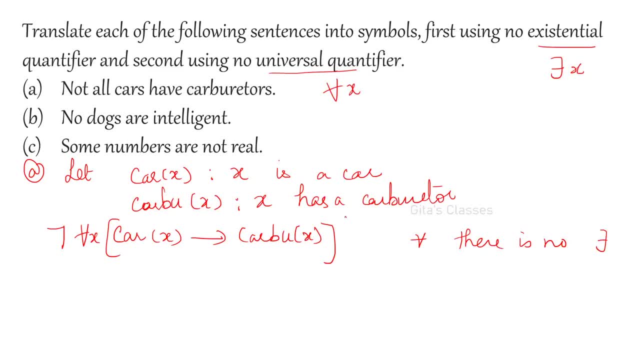 First form, There exists, is not there. Now the same statement you have to write without for all: You can have: there exists. Okay, what will you do? You take negation inside. We have for all x. no, Take negation inside. 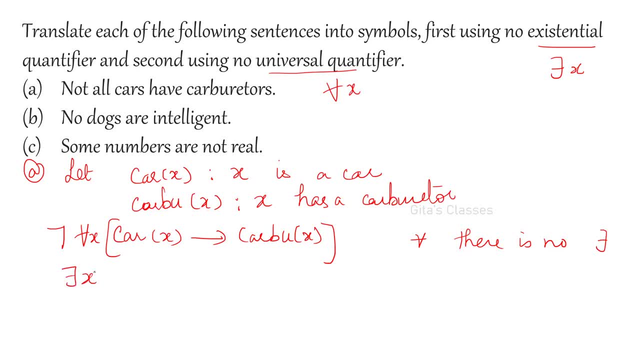 So for all x will become there exists x. If you take negation negating the statement there exists x, then negation of and this P conditional Q is what P conditional Q is equivalent to, not P or Q. This you have to remember. 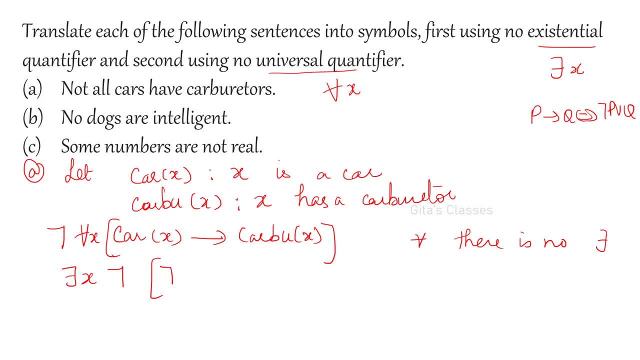 I told you throughout this unit, we will use this. So not negation of negation of car of x or carburetor of x. That is, there exists x. Now again, you take: this is using De Morgan's law. you have to apply. 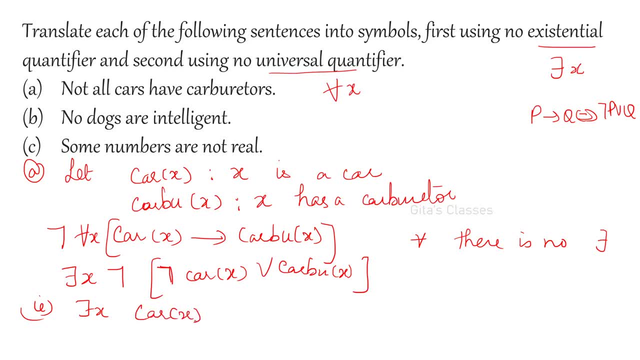 So negation of negation of car of x, it will become car of x right, And R will become, R will become, R will become. and then negation of carburetor of x. So there exists x. 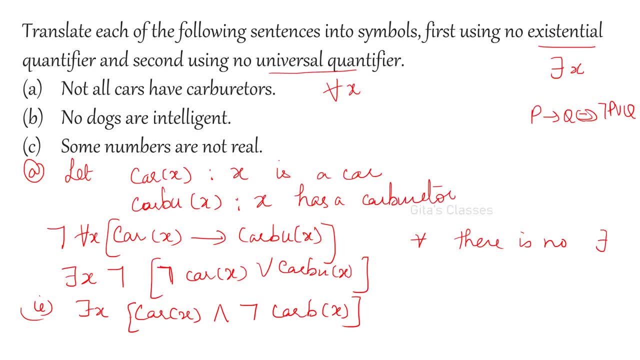 Here double negation will become car of x. Okay, So there exists x, car of x and not of carburetor of x, carburetor of x. So here we have: there exists, there is no. This is another one. 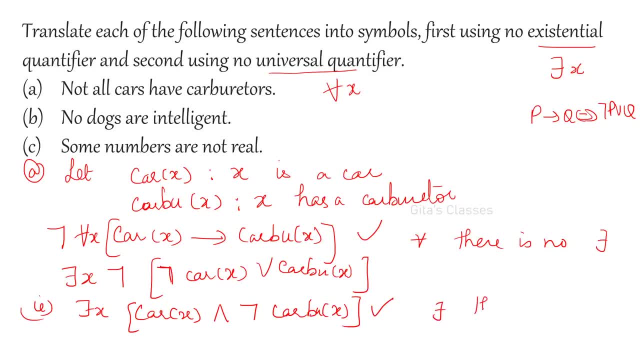 This is first form. second form: There exists, is there. There is no for all. Okay, So how will you write this? actually, There exists a car, but it does not have a carburetor. There exists a car which does not have a carburetor. 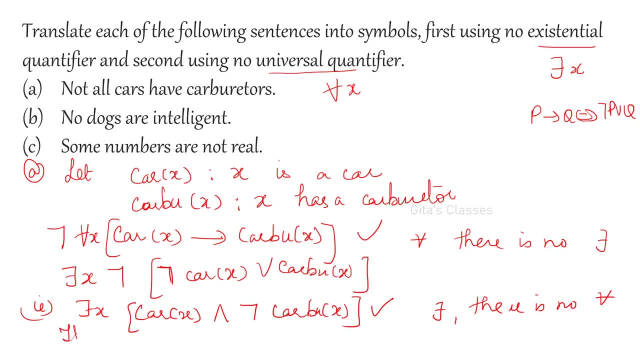 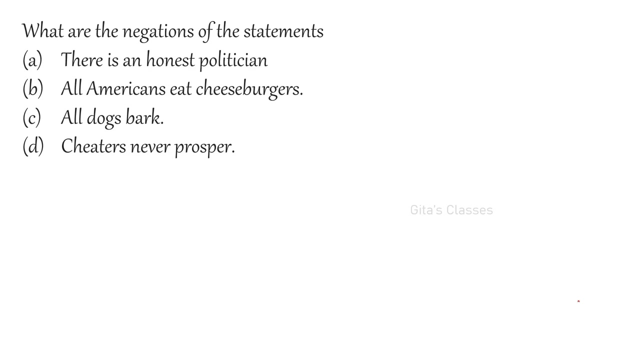 That is a statement here. If you want, you can write: There exists a car which does not have a carburetor. Okay, Next question: What are the negations of the statements? These kind of questions you can expect even for university exam. 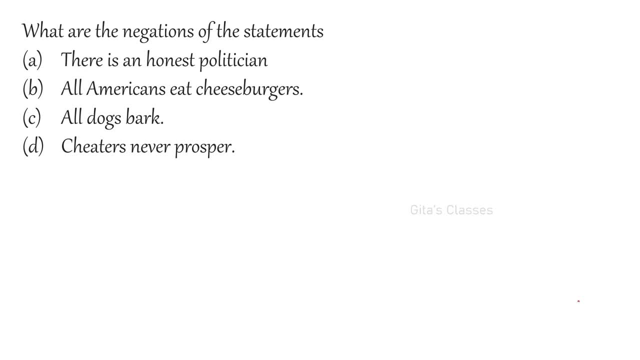 Some statements will be given. You will be asked to write the negation of the statements. So what are the negations of the statement? There is an honest politician. So first one, We will write h of x. h of x is x is honest. 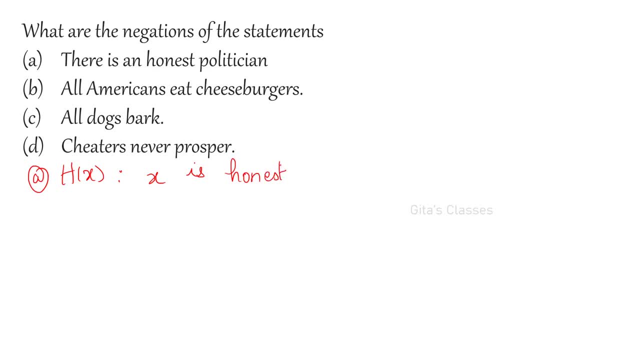 Always remember you have to write in terms of x and you have to write the domain also Here. what is the domain? Domain is the set of all politicians. Domain is the set of all politicians For one question. I will write everything remaining. you can follow that. 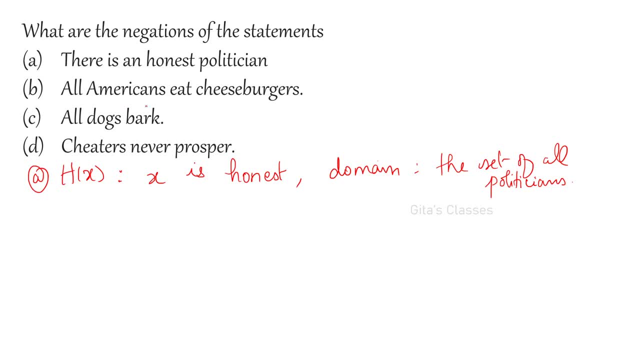 So h of x. x is honest. So what is the given? There is an honest politician, So there exists x. h of x. This is the given statement, right where the domain is the set of all politicians. right Now, how will you write the negation? 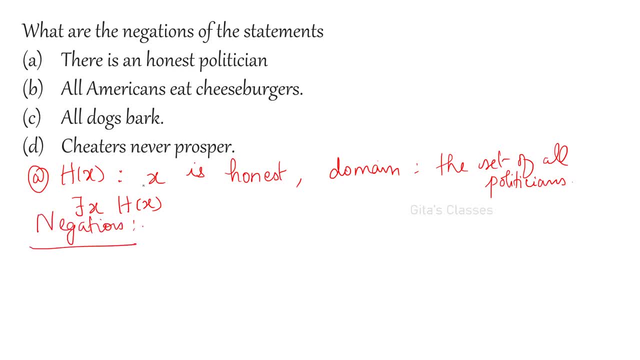 You are asked to write that this is the given statement you have written in the symbolic form. Please remember: whenever these kind of questions are asked, don't write exactly Without writing the symbolic form. don't write from the English. it will become wrong. okay, So there exists h of x. 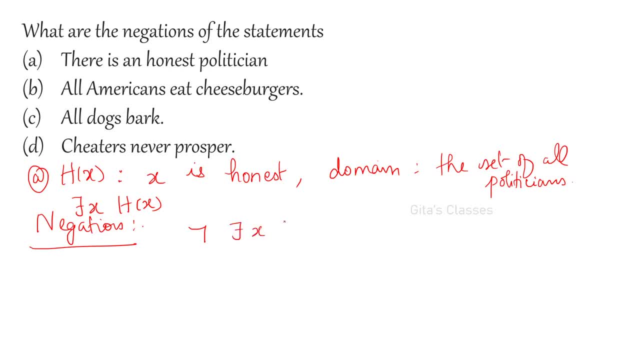 So negation. So negation means not of there exists x, h of x. So this is equivalent to: Now, if you want to take negation inside, there exists will become for all x, then negation of h of x. That means for all x, not of h of x. 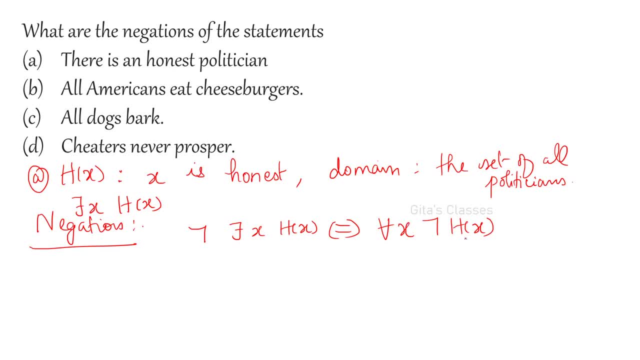 H of x is what X is honest. What is negation of h of x? X is dishonest or not honest. And for all x, that means Every politician is dishonest. Every politician is dishonest. Okay, So in English generally we say: all politicians are not honest. 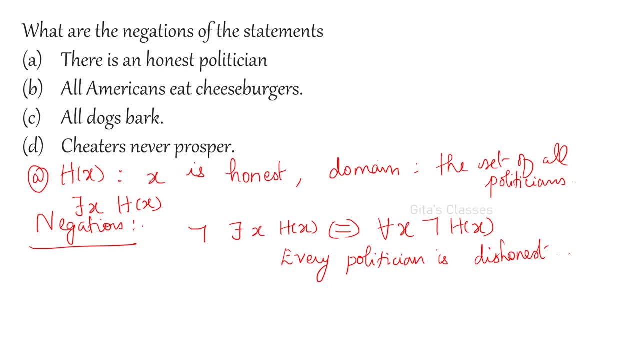 That may not. that is ambiguous, Okay, that will not give a clear picture. that is ambiguous, right? So not all politicians are honest and all It will be Giving different meanings, right? So second one: All Americans eat cheeseburgers, So b? 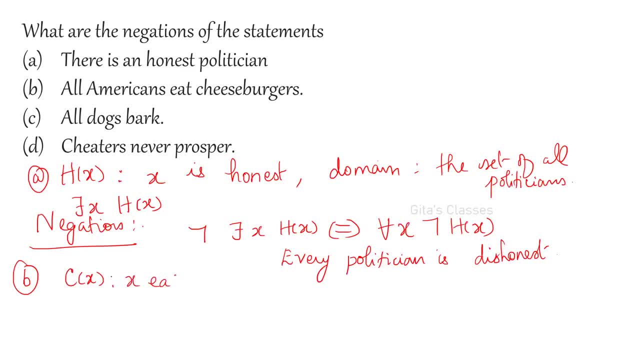 So let us write: c of x, X eats cheeseburgers, Not Americans. Indians are also eating, right? No? So c of x, X eats cheeseburgers. So what is the statement Given? all Americans eat cheeseburgers. So what is the? 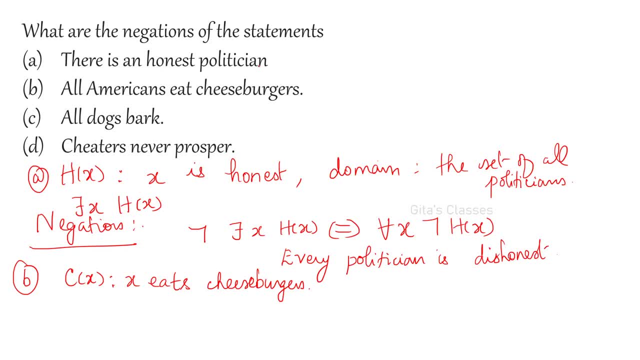 Here x eats cheeseburgers. Here the statement is: all Americans. Therefore, our domain is all Americans, Right? So what is the given statement For all x, c of x? For all x, c of x, Where the domain is: Domain consists of all Americans. 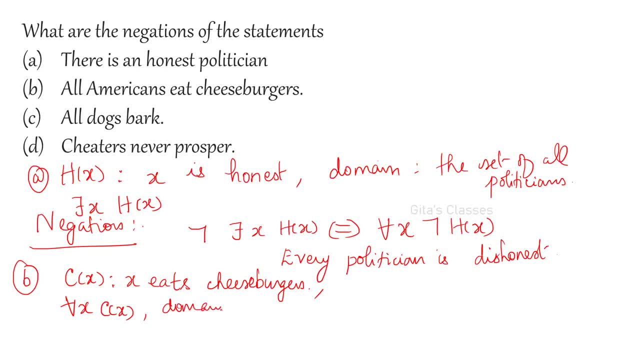 That is, the given statement Domain consists of all Americans. So How will you take the negation now, Negation of For all x, c of x, So for all x will become There exists? This is equivalent to For all x will become. 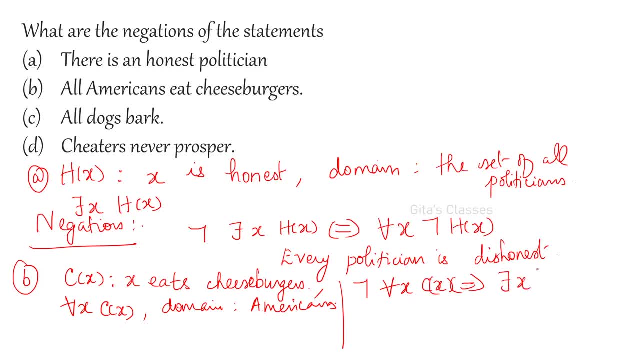 There exists x, Not of c of x, Not of c of x. That means what? There is an American Who does not eat cheeseburgers. There is an American, That is. there exists one x, So there is an American. 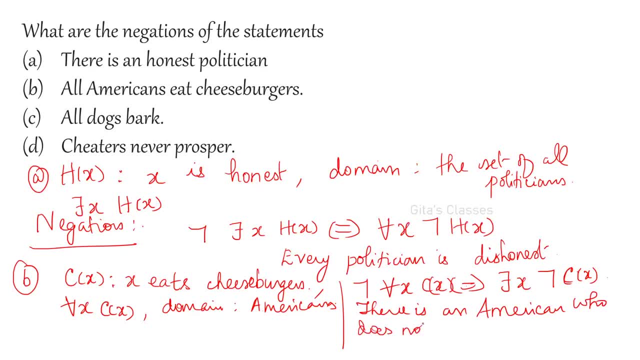 Who does not eat Cheeseburgers, Okay. Or You can say: some Americans Do not eat cheeseburgers. Also, you can say: Another way of telling is Some Americans do not eat cheeseburgers. That is the negation. 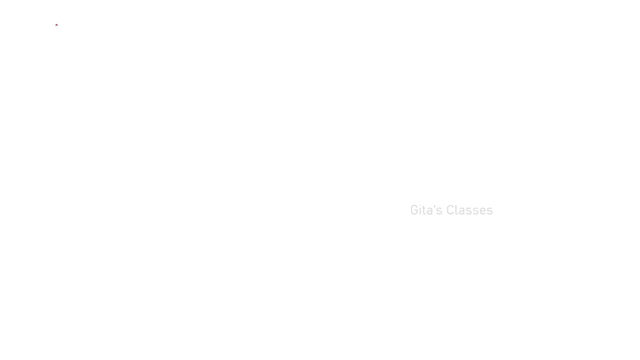 Next is: All dogs bark. So let us take p of x Where x barks. And what is the domain here? Set of all dogs. So what is the given statement? For all x, p of x, For all x, p of x. 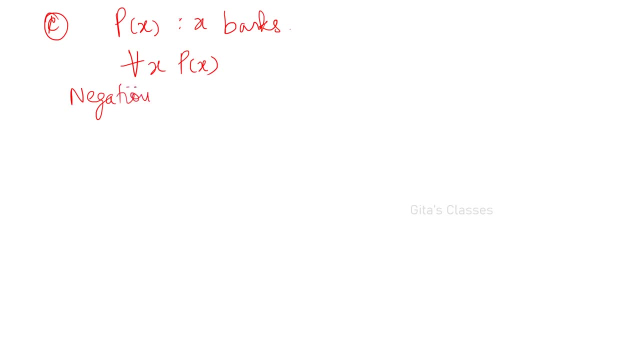 What is the negation? Take negation of For all x, p of x. It is equivalent to For all x will become: There exists x, Not p of x. What is the meaning? At least some dogs do not bark. 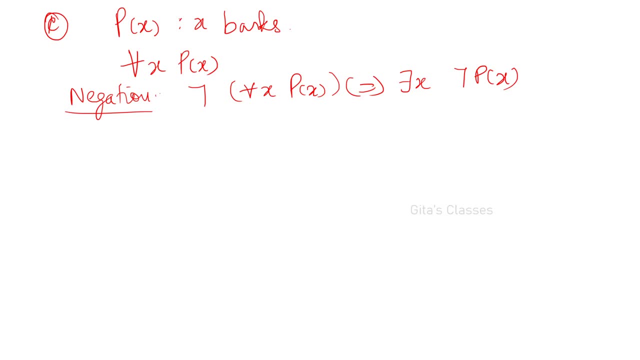 You can say: Or there is at least one dog Which does not bark- Some dogs Do not bark- Or you can say: There is at least one dog Which does not bark. Also, you can say Then d? What is the fourth statement? 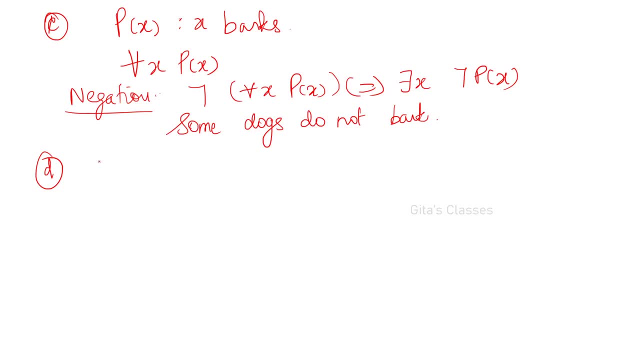 Cheaters never prosper. Cheaters never prosper. Let us say p of x, X never prosper, X never prospers. So here, What is the domain Set of all cheaters, Right? So what is the given statement? Cheaters never prosper. 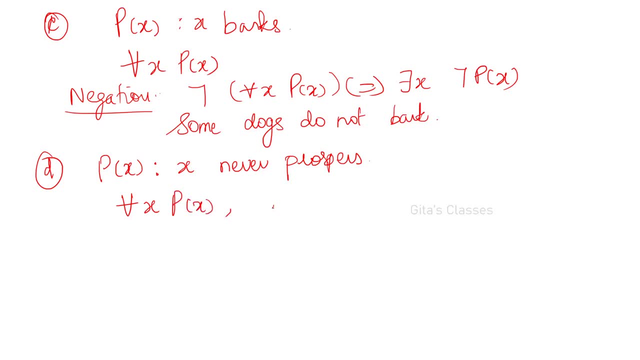 So for all x, p of x, Where x takes the domain is The set of all cheaters, Set of all cheaters. Now, what is the negation? Negation is Not of For all x, p of x. That is equivalent to: 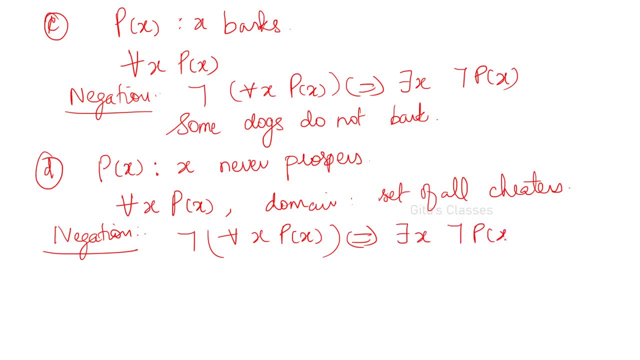 For all x will become. There exists x, Not Not of p of x, That is, There exists a cheater Who Prospers Never Here. x never prospers Means It is, They don't prosper. 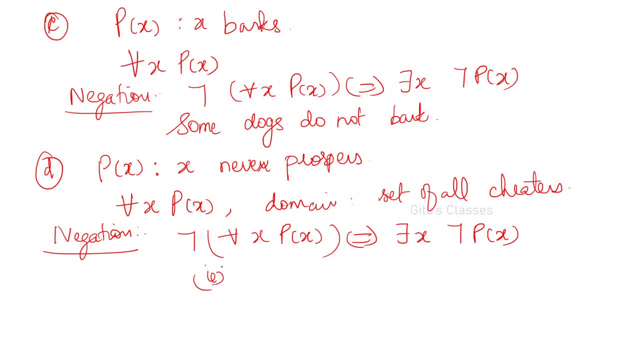 But here Negation is They prosper. Okay, So there is At least. There is a cheater Who prospers. There is at least one cheater Who prospers, Who prospers. You can say like this: or some cheaters prosper also. you can say: some cheaters prosper. as we have written in the third sentence, some dogs do not bark in the same way here. some cheaters prosper also. you can see some cheaters prosper. 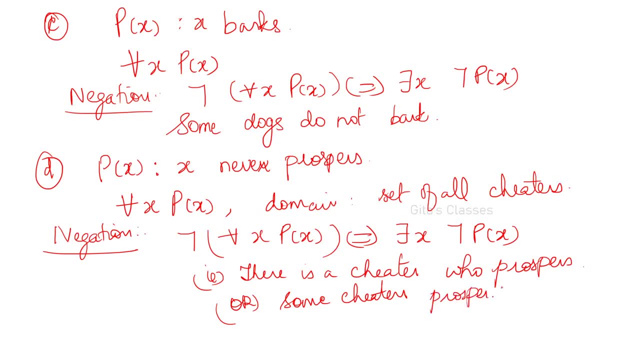 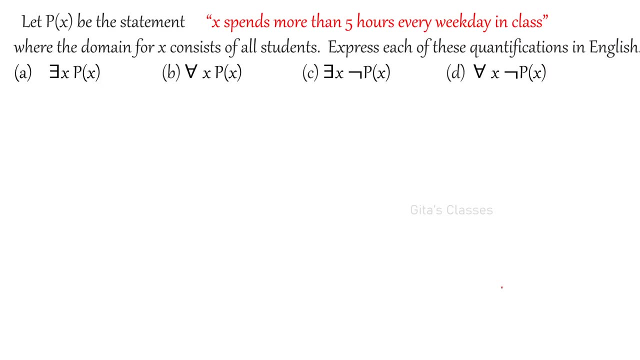 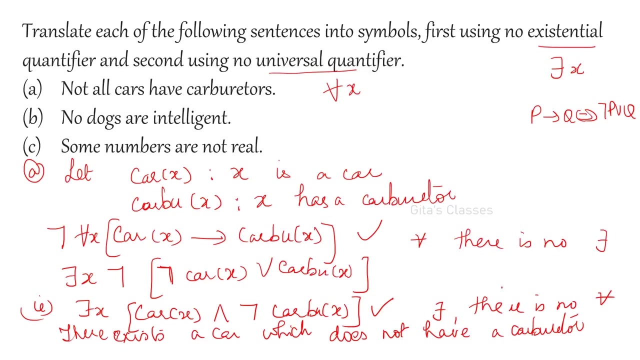 So let p of x be the statement. The next question: that p of x be the statement. x spends more than five hours every day in in class, every day in class. I think we have left two questions here. no, dogs are intelligent. some numbers are not real. that also will do after this. okay, so let p of x be the statement. 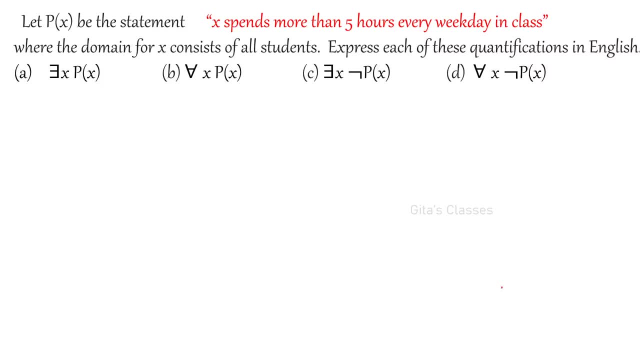 Let p of x be the statement. x spends more than five hours every day in class, every day in class, every day in class. So let p of x be the statement. x spends more than five hours every day, every weekday, in class. where the here till now English sentences were given, we have written in symbolic form and take the negation and all now symbolic form is given, you are asked to write in the English sentence where the domain for x consists of all. students express each of the these quantifications in English. 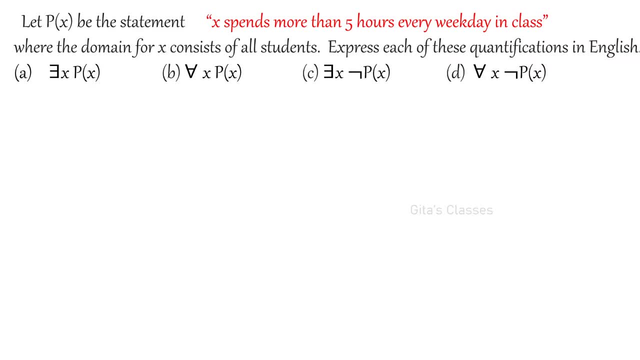 So first one is: there exists p of x. What is the statement? p of x? P of x expense more than five hours every week day in class. okay, there exists x. p of x means what: there exists at least one student who spends more than five hours in every five hours every weekday in class. 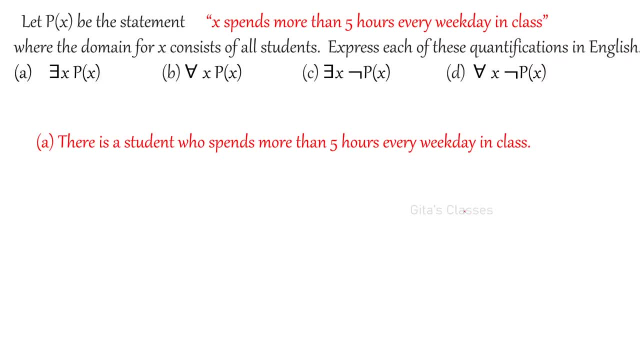 So there is a student who spends more than five hours every weekday in class. whatever is the given sentence you write, as it is only for this, you have to be careful. there exists at least one student. So there is a student who spends more than 5 hours. Now for all x, p of x. that means what every student is. 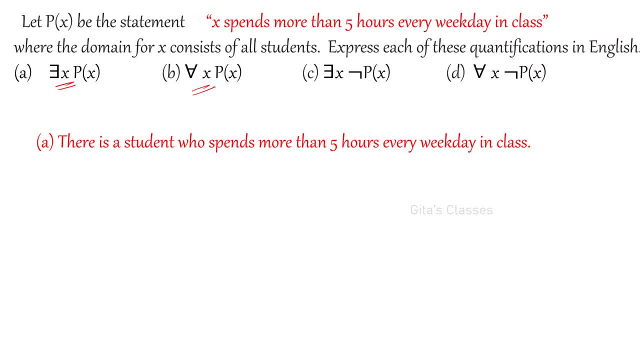 spending may have more than 5 hours every weekday in class. right for all x, p of x. So every student spends more than 5 hours every weekday in class. and one more thing next is: there exists x who is not spending, so negation of p of x. P of x is expense more than 5 hours. Negation means what? 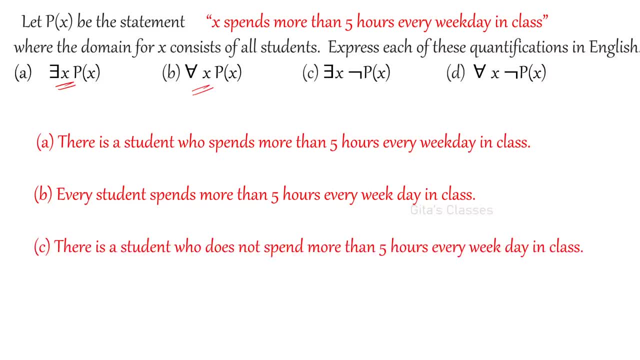 they do not spend. So here there exists a student. there is a student who does not spend- okay, you have to write that- who does not spend more than 5 hours every weekday in class. The same thing here also. no student is spending 5 hours every day. okay, that means no student spends more than 5 hours. 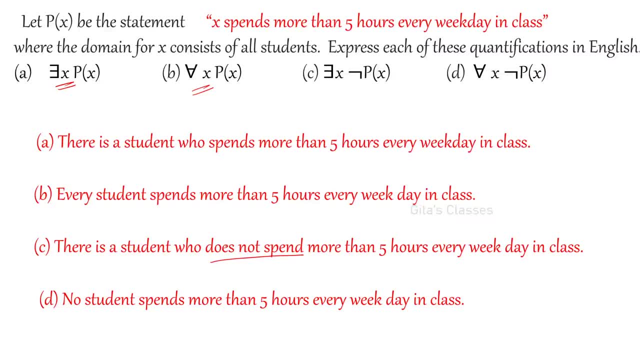 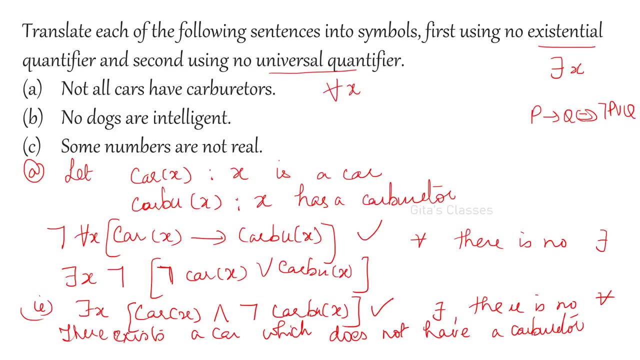 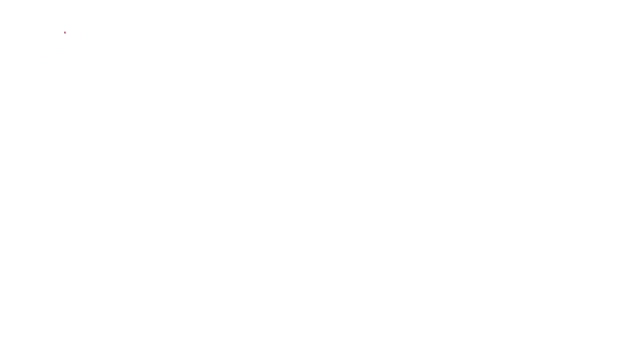 every weekday in class. okay, Next is these two. I will give you the answers. you can, you can, you can no, dogs are intelligent. Here I will do wait. No, dogs are intelligent. that means here dog dog a of x, b dog of x. let us take: x is a dog. 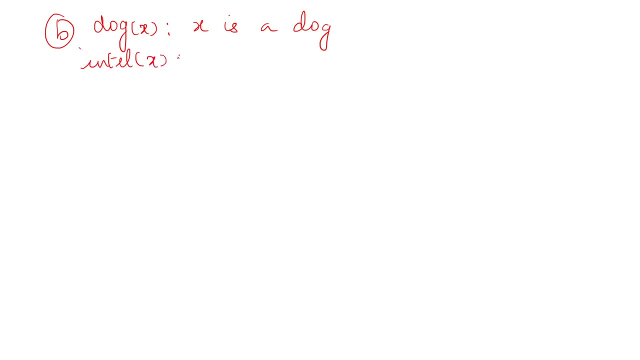 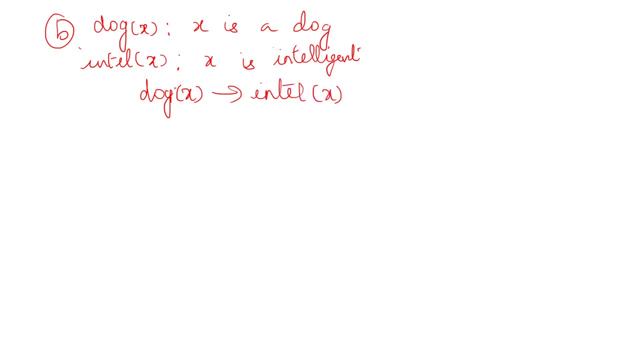 intelligent, So intelligent of x. So for all x. if you take any dog, it is not in. no dogs are intelligent. So for all x, if it is a dog, it will not be intelligent. So here we have. we have used for all there exist is not there. This is one form. Now we have to use negation. sorry, there exist, but you should not have for all. So now we from this. what we have to do is take double negation. Introduce here already the previous question, negation. 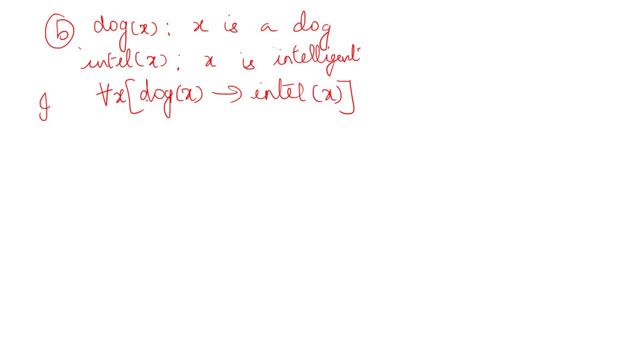 Negation was there, so we have taken inside Here. negation is not there because we have to change this for all to there exist right. How is it possible? Only by negation. Here no negation is available. therefore, I am taking introducing two negations. 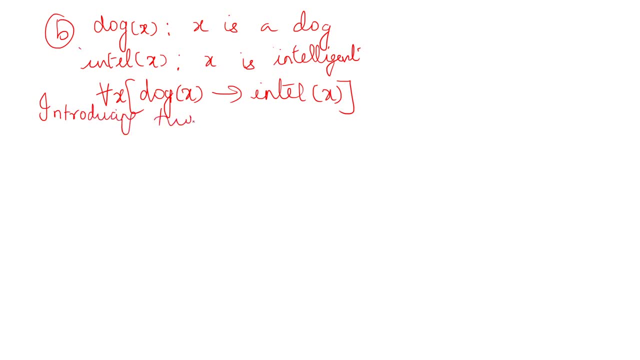 Two negations. So. negation of negation of for all x. Negation of negation of this is P conditional R, P conditional Q means P R, wait, wait here. negation of intelligent: If it is a dog, it is not intelligent. So we will have 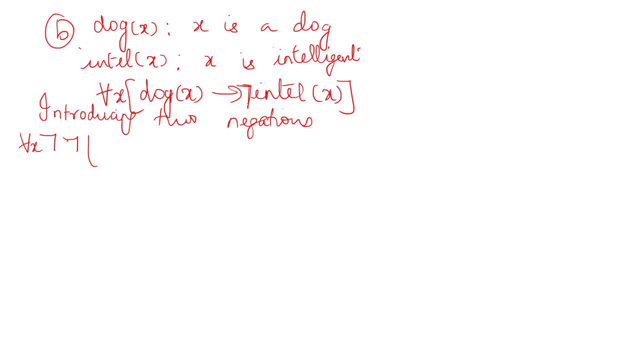 one more negation here, Negation of intelligent, So P conditional Q means not P R Q, So not of dog of x R, not of intel of x. Okay, Now you bring one negation to the to before and one negation after, So. 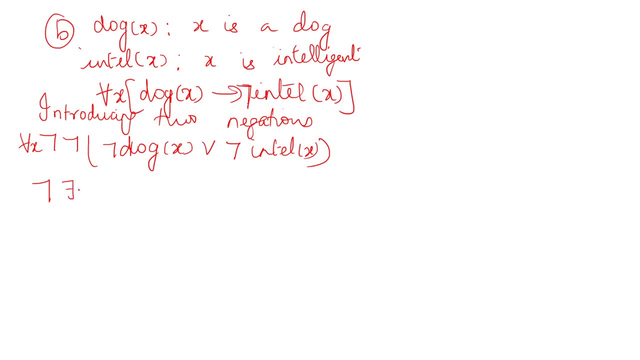 negation of this, for all x will become. there exist x right. Then one negation: you take it inside. So negation of negation of dog, of x right. Already we have one negation. This negation I am bringing to the this side, bringing to the left hand side, and here, 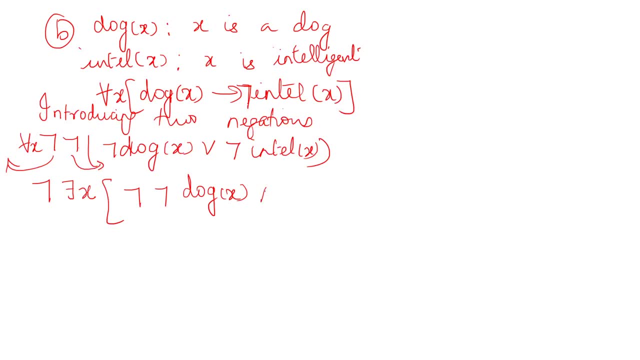 I am taking inside. So negation of negation of dog x. then here again, one more negation: we have intel of intelligent of x. This is equivalent to negation of there exist x dog, of x and intelligent of x. So there exists a dog where it is a dog and intelligent, which is not possible. So negation of there exists at least one. There exists x dog. that is nothing is available like that Here there exists. without this negation. if you remove this negation. there exists a dog which is intelligent Here, it is not true that it is no such entity is available. Okay. So negation of there exists at least one. There exists x dog. that is nothing is available like that Here there exists. without this negation. if you remove this negation. there exists a dog which is intelligent Here, it is not true that it is no such entity is available, Okay. So negation of there exists at least one, There exists x dog. that is nothing is available like that Here there exists. without this negation. if you remove this negation. there exists a dog which is intelligent Here, it is not true that it is no such entity is available. Okay. So negation of there exists at least one. There exists at least one. There exists x dog, that is. nothing is available like that. 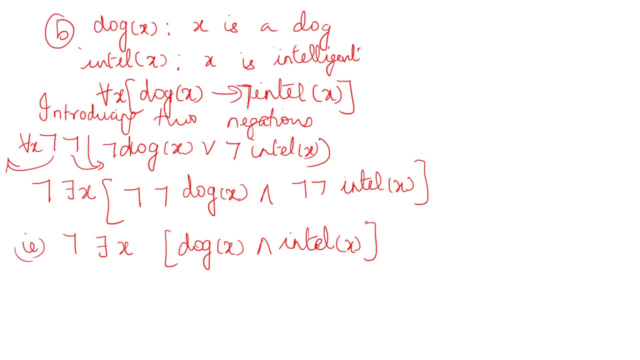 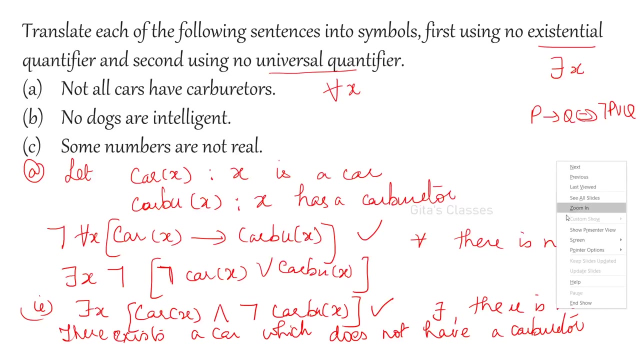 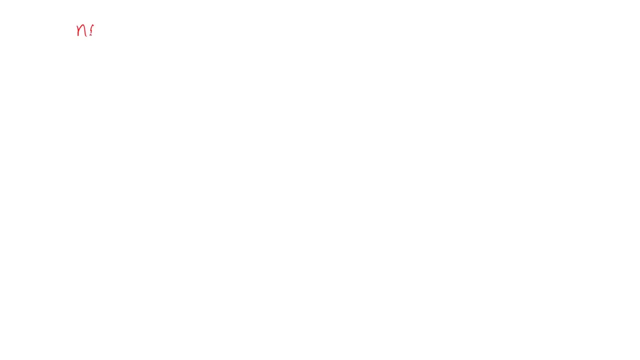 Okay, That is the meaning. Next is: some numbers are not real. Some numbers are not real. Some numbers are not real. So that means let number of x, number of x is x is a number, x is a number and real of x always. you try to write them in the 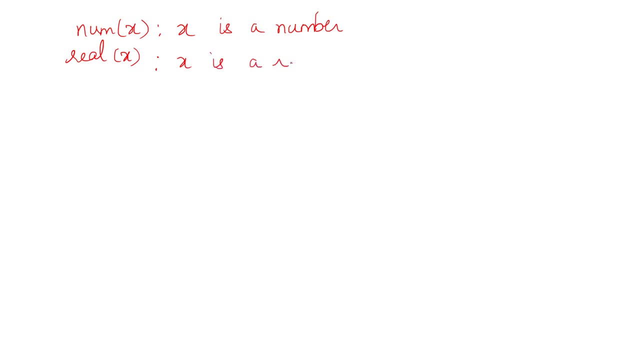 atomic form. Okay, So x is a real, x is real. So what is given? There exists a number, x- and not real. Some numbers are not real, So not real of x. There exists at least one number, x, such that it is a number and not real. 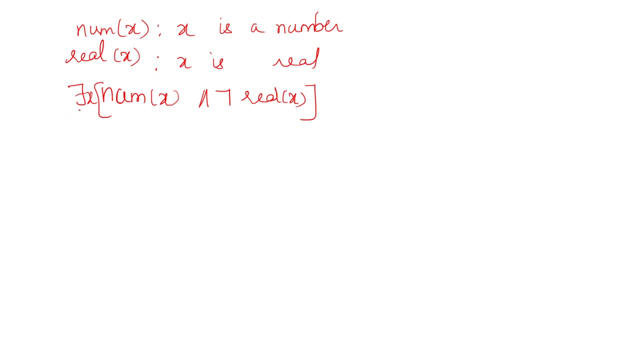 Okay, So here we have used there exists, but there is no for all. Now we have to bring it to for all. there exists should not be there. Okay, The other form. We are asked to write in both the forms. So here, introducing: